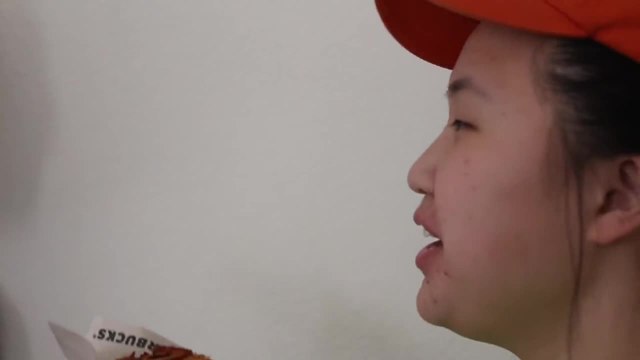 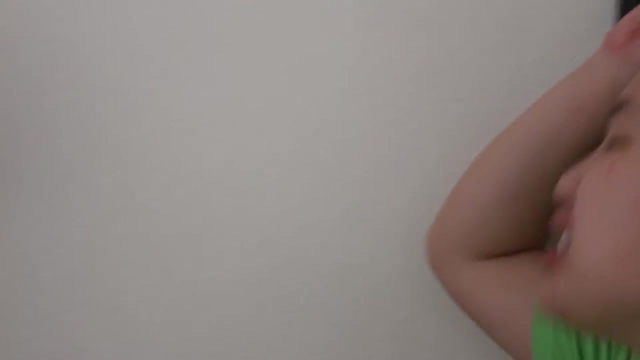 HanyuMany, we need you to make the World Cup Stadium Sure, And I can use the Pythagorean Theorem to measure out the wood. I guess, Boss, Boss, I finished the stadium for you. I asked for a real building, not there. 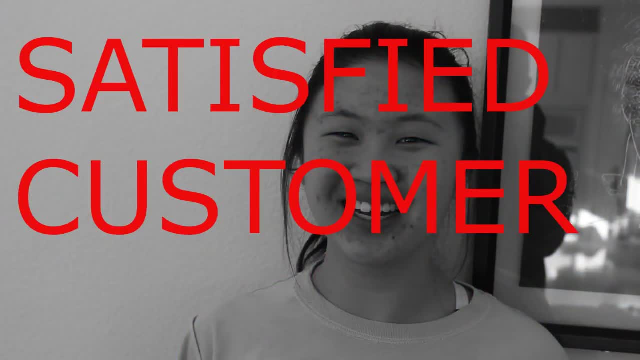 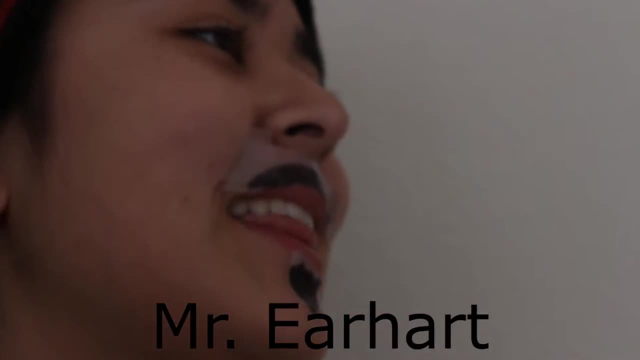 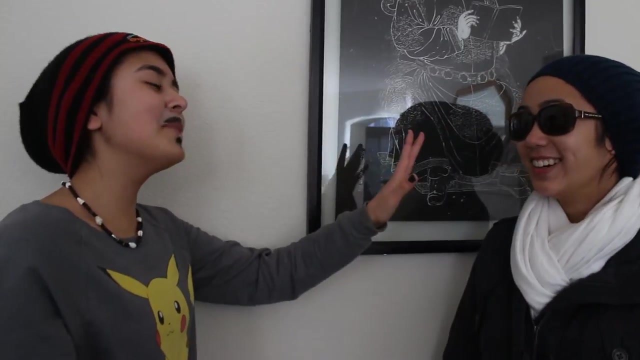 Thanks, Trigonometry. Amelia, I need you to fly around the whole entire world. Only then I, your father, will be proud of you. But, Daddy, I just need a break. I just I'll be seeing you Now, time to make a 360 degree turn and get out of here. 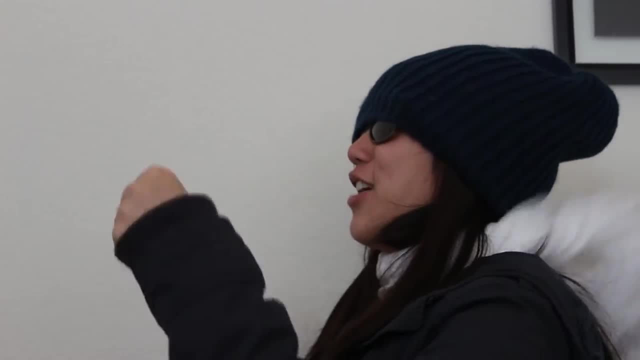 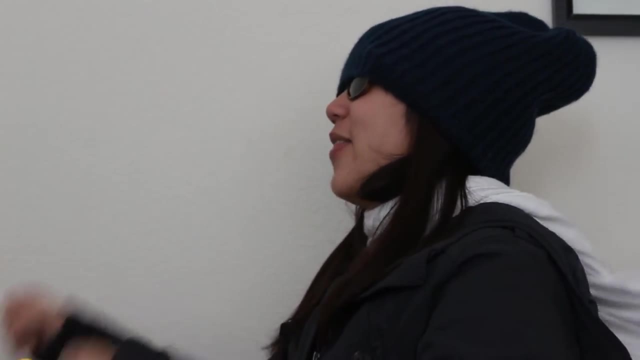 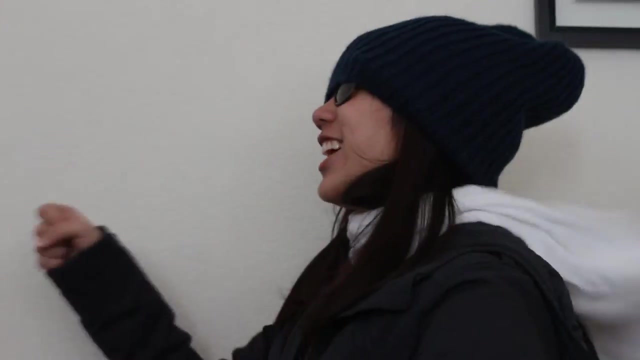 I can use Trigonometry to determine the trajectory of my flight path And, using right angles, I can determine how high I will rise over a certain object. And then I can use my angle of depression with my bearings and rise down safely without crashing. 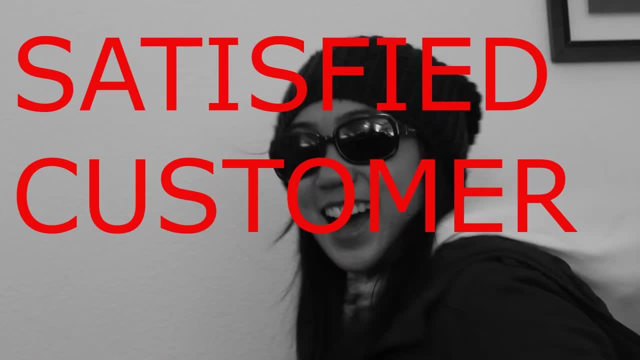 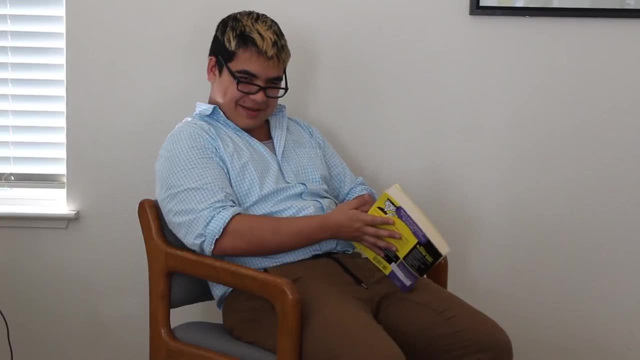 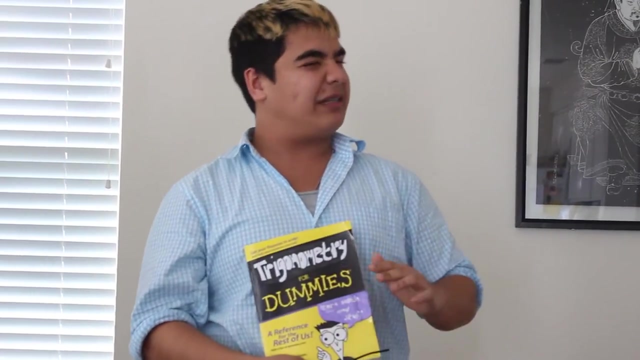 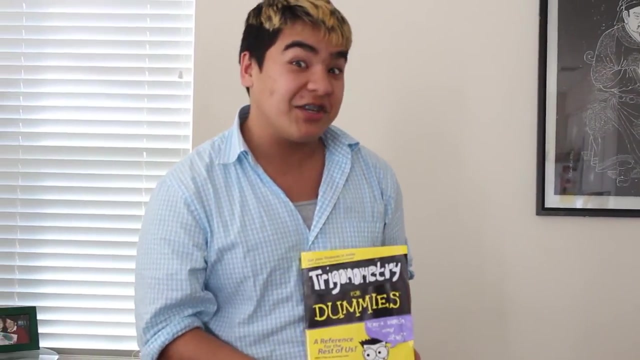 Thanks, Trigonometry Host. host, we're rolling. I didn't see you there. I was busy reading Trigonometry for dummies. You see, all those customers were completely satisfied with the course we gave them. Now we're going to give you a look into what our course has to offer. 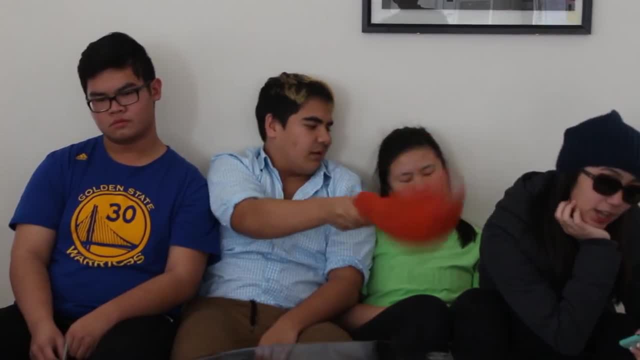 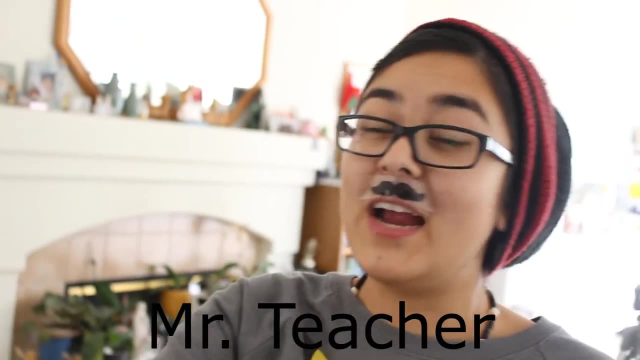 I can't believe that guy took the 30- Quit sleeping Pee-wee. Touch a lamp. Uh, uh right, uh uh. Trig, Trig. let's get back to Trig Teacher. Yes, host. 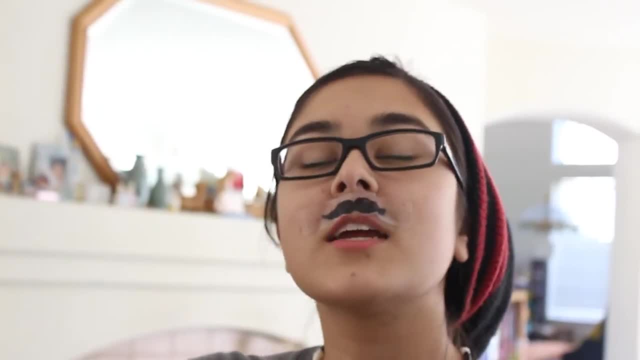 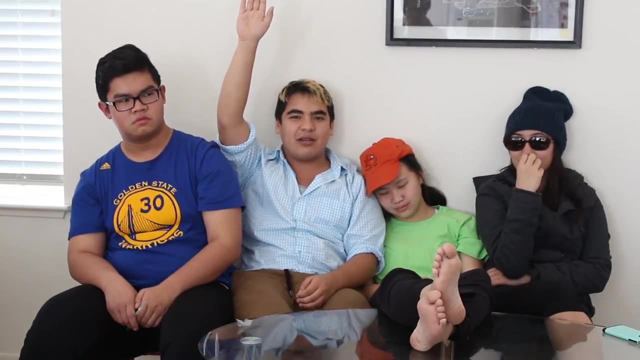 Can I use the bathroom teacher? And how does that use Trigonometry? I use right triangles to count each tile on the way to the bathroom teacher. So 45 degree angle means I take the bearings south to east teacher. 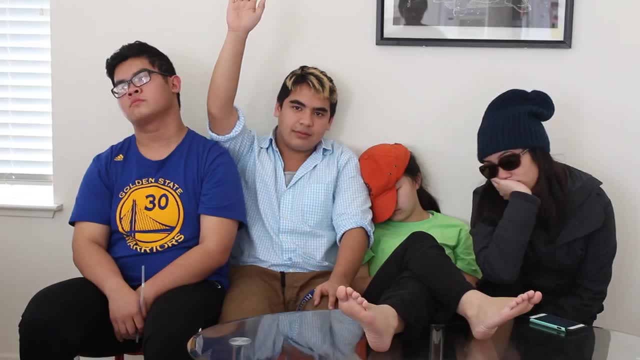 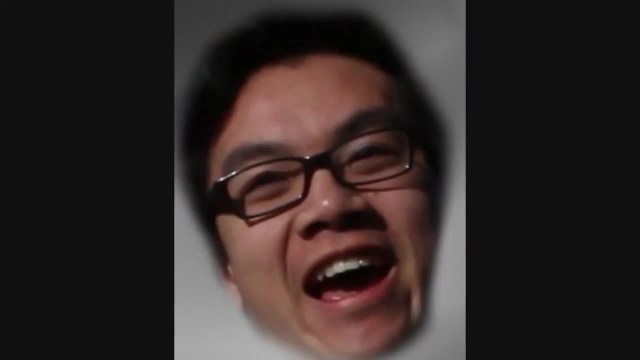 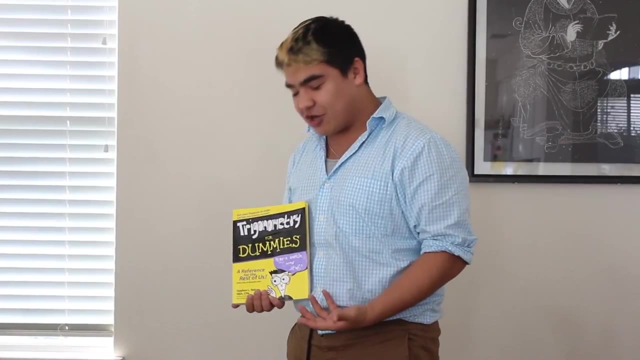 I just just just just go use the bathroom, kid. Thank you, teacher. Professionals from all across the world use Trigonometry And you can use Trigonometry just like them If you take our course Trigonometry for Dummies. 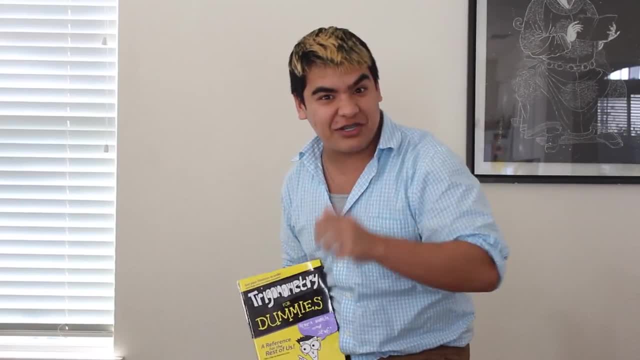 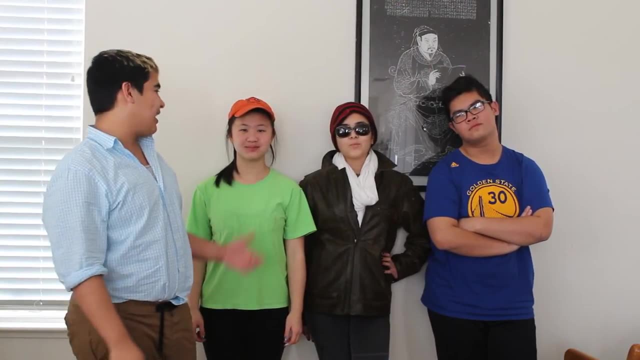 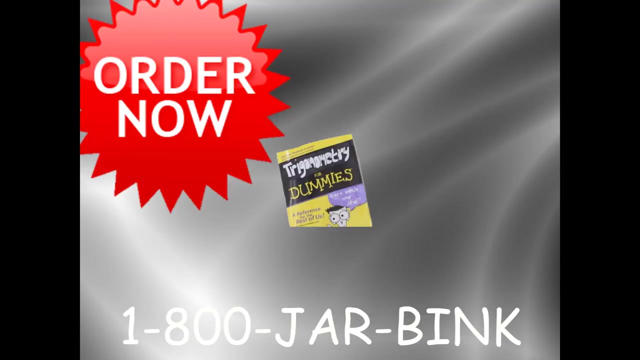 all you have to do is give us cosine of 360 payments of $13.99.99.. Then maybe one day you too could be like Handyman Amelia Earhart or even Jose Curry. Order your novel of Trigonometry for Dummies today.